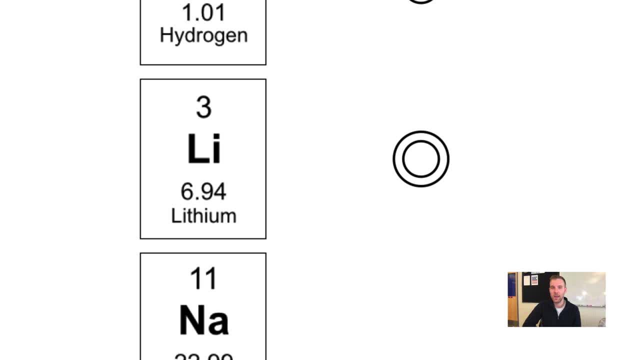 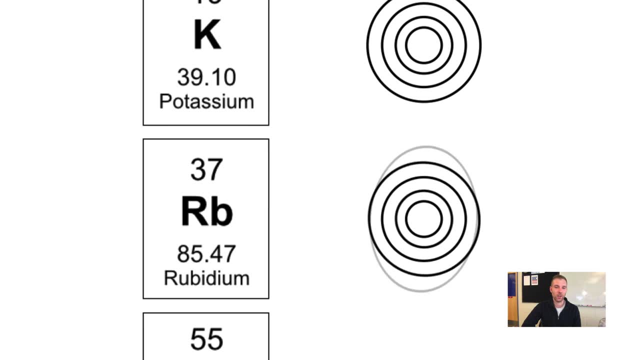 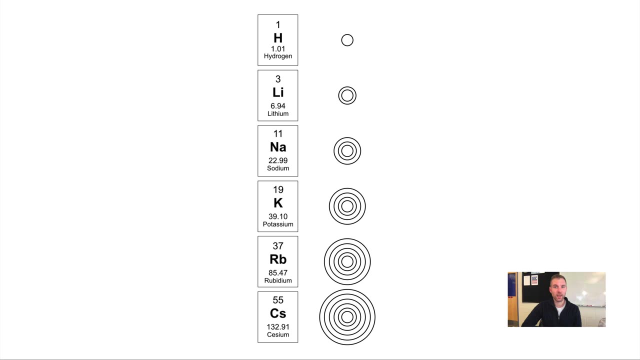 will have to go into the second shell. So lithium has two shells And as you kind of go from top to bottom in this group, we see that we just have an increasing number of electron shells Because the electron amount is going up and we need more room to house those electrons. the way that we house 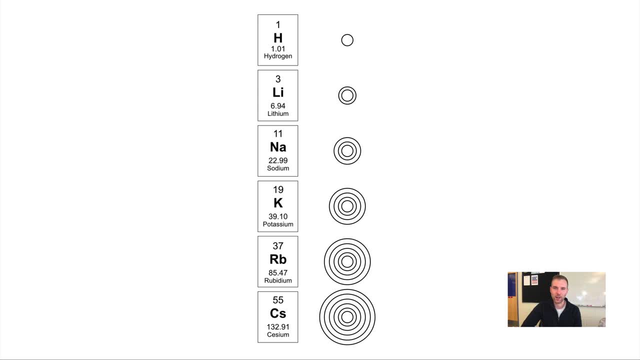 those electrons in an increasing amount is by just bringing in more electron shells to hold them, And what you can see is that as we go top to bottom, there is a bigger radius because we have more and more electron shells. The way to remember this just quickly is to think of a snowman, If you look at 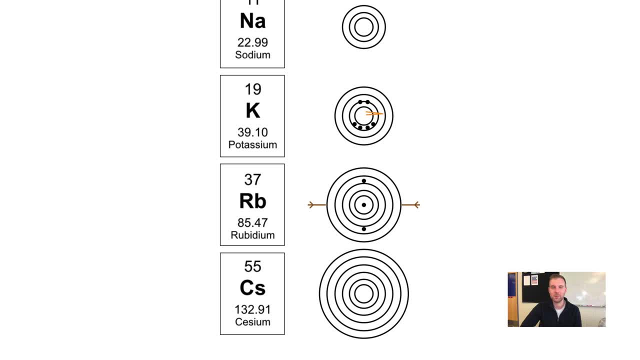 these bottom three. here you see a snowman. That was always my trick for remembering this, and I'm sure it's plenty of other people's too. It can be yours, but the reason that that's happening is because there are more and more electron shells as we go from one period to the next down a group. 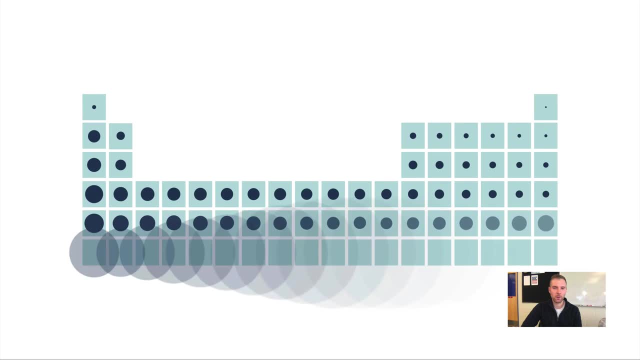 Now let me lay out the picture for you. I'm going to show you a picture of a snowman. I'm going to see if I can put my hand over the thing here. In this case, I'm going to place a snowman. I'm going to 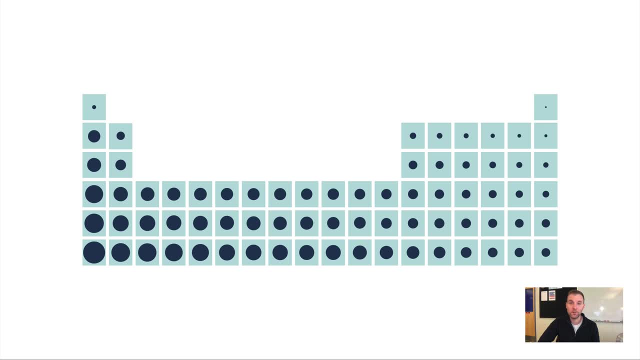 capture it in a little picture. I'm going to place the snowman on top of the snowman. Let me see if I can copy that. Okay, so we have the atomic radius for all of the elements on the periodic table. What we see is that top to bottom trend of the atomic radius increasing. But what you'll also see, 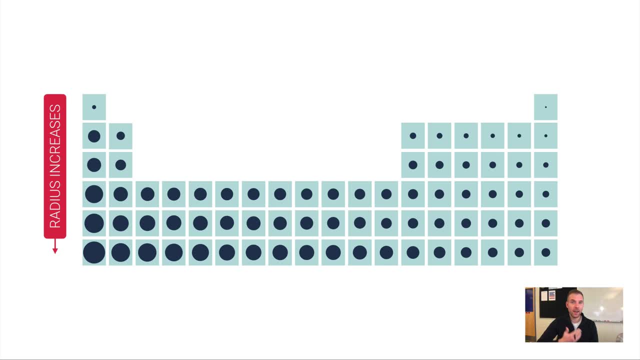 is that as we go from left to right, within a period the atomic radius actually decreases. Now that may seem strange to you, because if we're adding electrons as we go to top to bottom and that's causing our radius to get bigger, shouldn't our radius get bigger as we go from left to right? 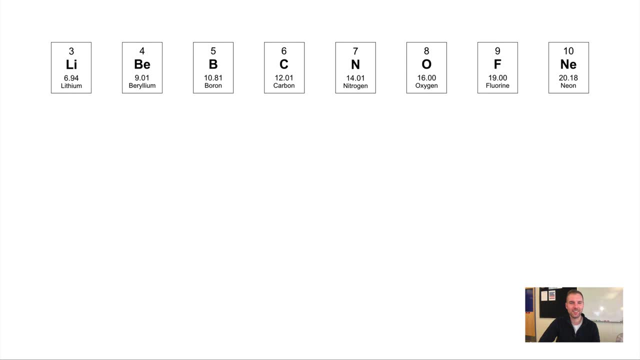 in a period. The explanation for this one is a little more complicated, so let's just take a look at the elements in period two: lithium to neon. Lithium has three protons and three electrons. As I slide over from lithium to neon, I'm adding one more proton, but I'm also adding one more electron. 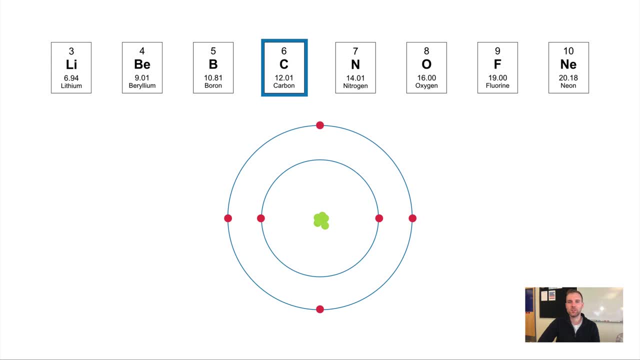 And as that happens the attraction of the electrons to the nucleus becomes greater and greater and that causes the entire electron cloud to just kind of scooch in closer to the nucleus. So you can see, of this grouping here, neon is actually the smallest atom and lithium is the biggest atom in period two. 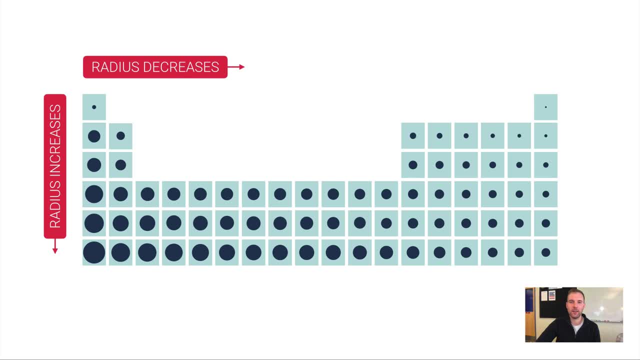 So now we have our full trend here. top to bottom, in a group, The atomic radius is going to increase. Think of the snowman effect there The radius actually decreases as we go from left to right within a period. So the overall trend. if you think of it this way, this may help you. 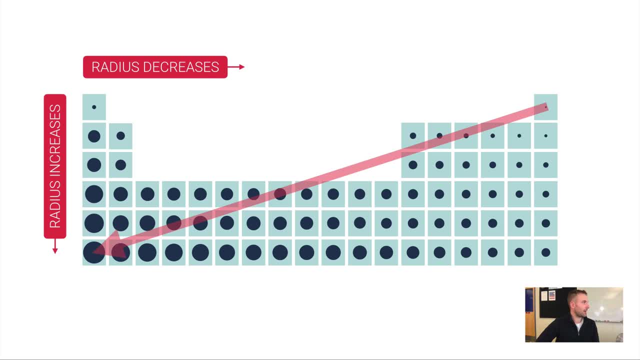 Helium is the smallest atom and francium- or I guess cesium, that would be on this slide here, but francium is the largest atom And so, knowing this trend, you can actually get a lot of the information for the other two properties we're looking at. 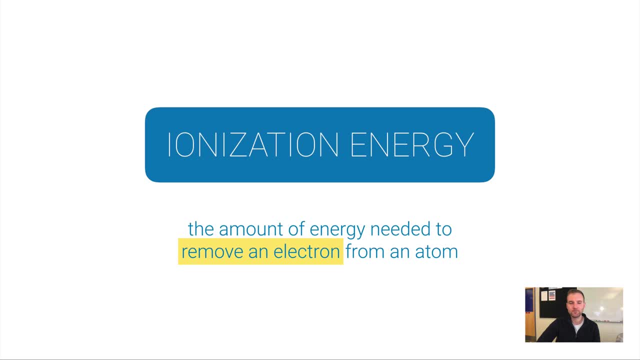 Ionization energy is the next property we'll investigate. Ionization energy has a fancy name, but it actually is not all that fancy when you know what it is. Ionization energy is the next property we'll investigate. Ionization energy is the next property we'll investigate. 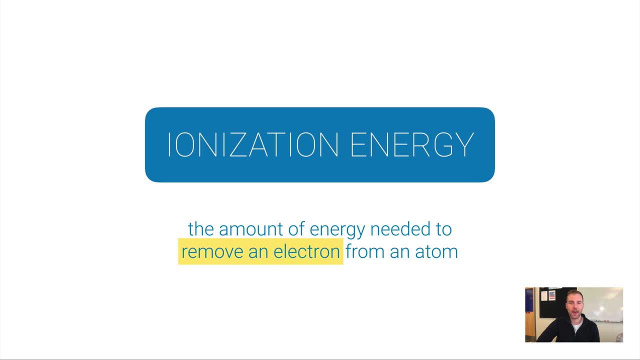 Ionization energy is the amount of energy needed to remove an electron from an atom. You can think of this almost like it's the cost of taking an electron from an atom. A low ionization energy means it's really easy to take an electron from that atom. 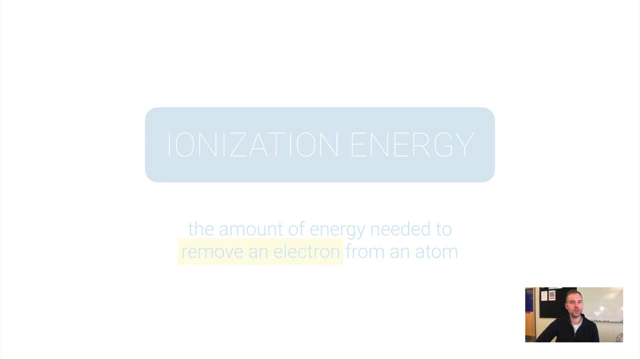 A high ionization energy means it's more difficult. Now here's the overall idea: The smaller an atom is, the harder it is to remove an electron from it. If I just look at an extreme case where I have a small atom, the valence electrons are really close to the nucleus. 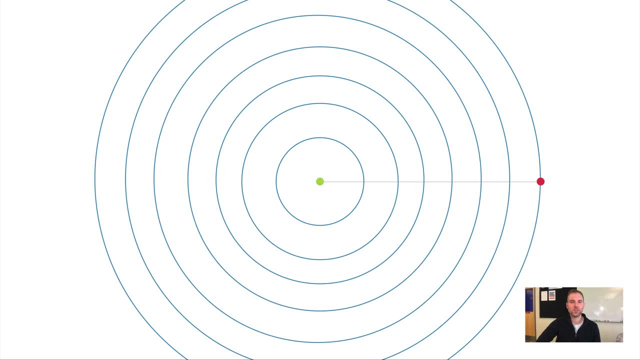 in this scenario. But if I have a larger atom, the valence electrons are much farther away from the nucleus and therefore they're much more willing to kind of be donated to somebody else. Another effect that's going on here is the fact that we have all of these rings that contain electrons already. 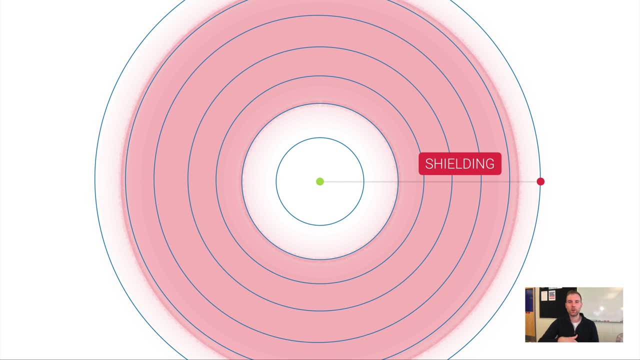 And so this is called shielding. Shielding is where the interior electrons kind of mitigate the attractive force of the nucleus, the outside valence electrons So said differently. The signal is kind of being blocked by the middle electrons, And so the valence electrons are not as loyal to the atom. 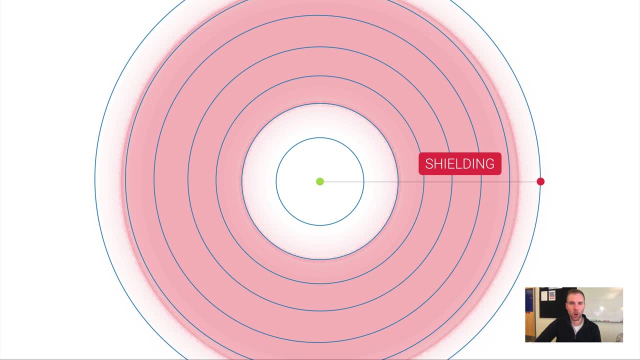 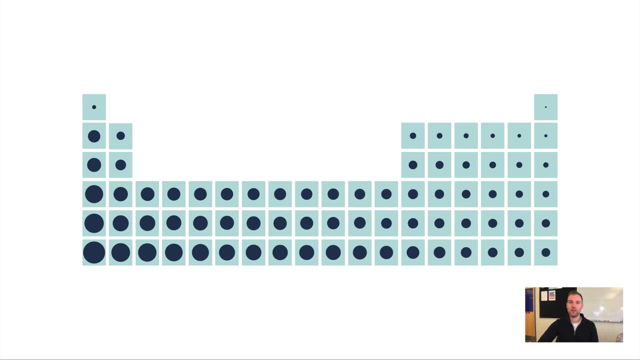 And so it's much easier to steal from a bigger atom as compared to a smaller one. Now, if we know the trend in atomic radius in the periodic table and we know that the bigger the atom is, the easier it is to steal from it, 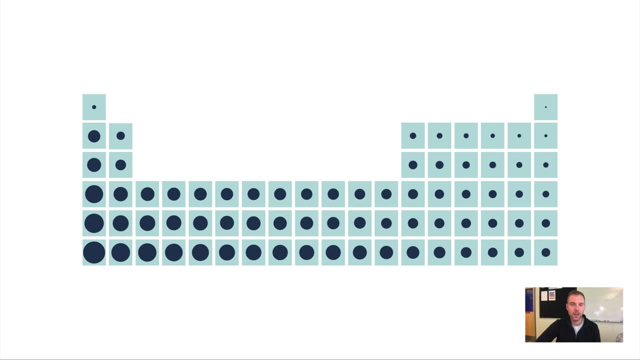 and therefore the lower ionization energy is required. then we can figure out what the trend in ionization energy would be. just based on knowing the size of the atoms across the periodic table, The ionization energy is going to increase from left to right. 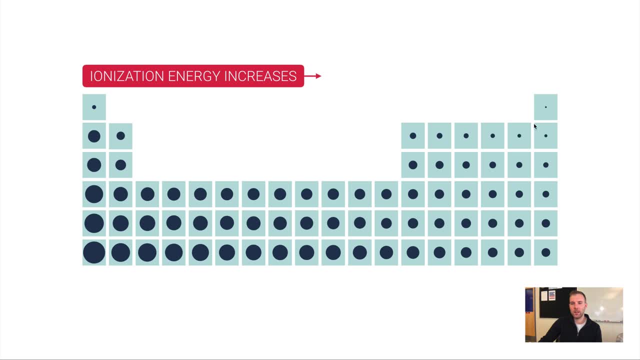 because if you just compare the size of lithium, for example, to the size of neon, this is much more difficult. So higher energy over here. because the size is smaller, Those electrons are being held really tightly to that nucleus- Lithium not as much as neon. so that means lower energy over this way. 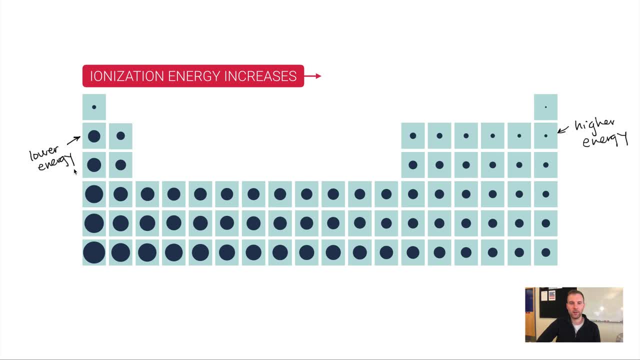 And remember, the lower the energy, the higher the requirement, the easier it is to take an electron from that particular element. If we know that from left to right across a period, and it's really just based off of the size, then we can also figure out what the pattern is from top to bottom in a group for ionization energy. 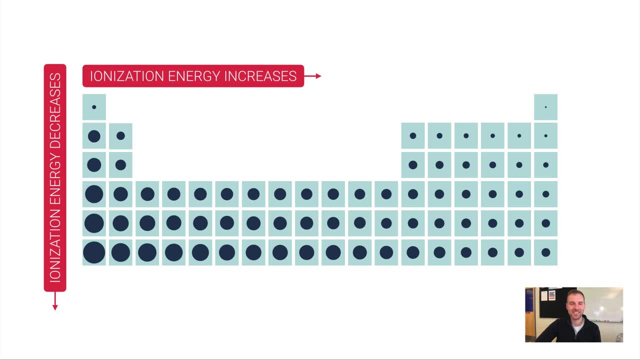 It's that the ionization energy decreases. So again, the bigger the atom, the easier it is to steal from it, and that means the lower the ionization energy will be. Okay, so the last piece is going to be electronegativity. 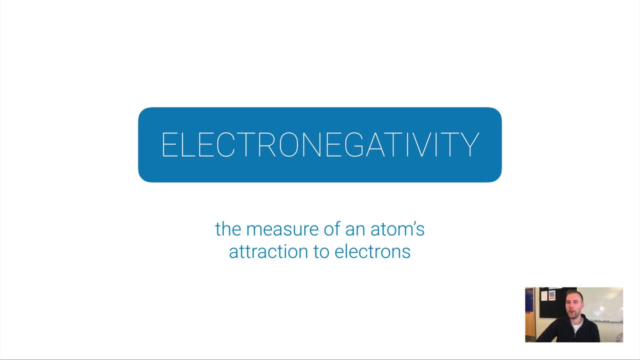 Electronegativity is going to come back when we talk about bonds and bond types. So this is something that is certainly important to know. It's going to help you when we talk about bonds, But in electronegativity what we're talking about is how much an atom wants an electron. 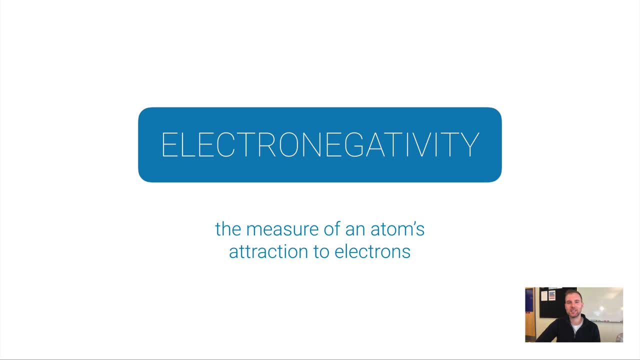 So it's a measure of an atom's attraction to electrons, and it's based on a scale from zero to four, where four is the element that really really wants electrons and zero is an element that really really does not want electrons. 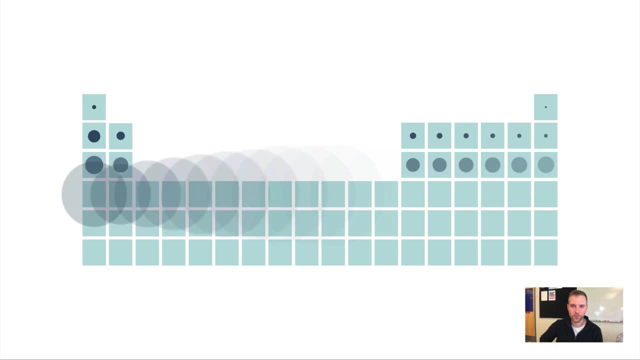 So let's look back at the periodic table. We fill in all the atomic radii for each of the elements here. I'd actually just like to look at kind of the two extreme scenarios here. Let's compare lithium to fluorine. Fluorine has seven valence electrons. 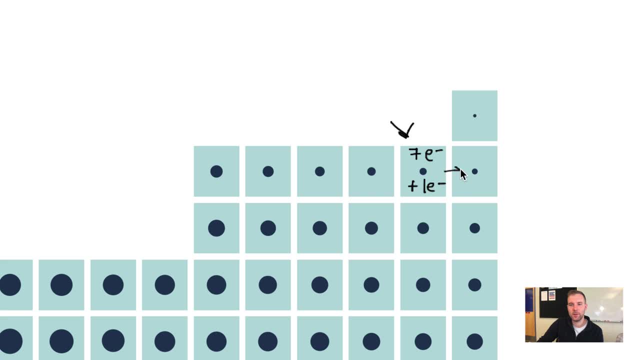 If fluorine can just gain one more valence electron, it'd be a lot like neon and that would fill its valence shell. It would satisfy the octet rule and fluorine would absolutely love to gain an electron. So fluorine's electronegativity is going to be really high. 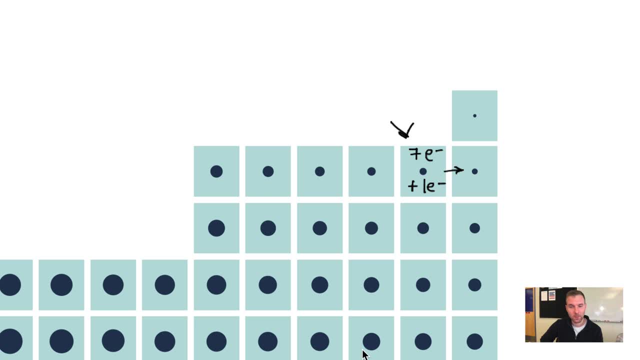 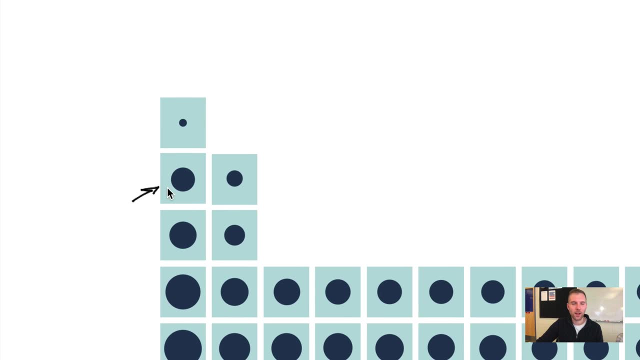 In fact fluorine has the highest electronegativity of all the elements on the periodic table. Now contrast that against lithium. They're in the same period but lithium is on the other side of the periodic table, the left side. 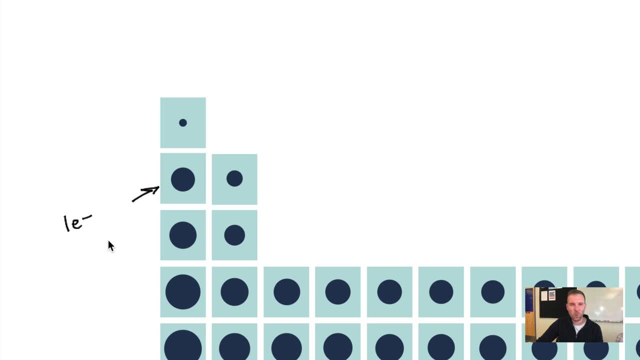 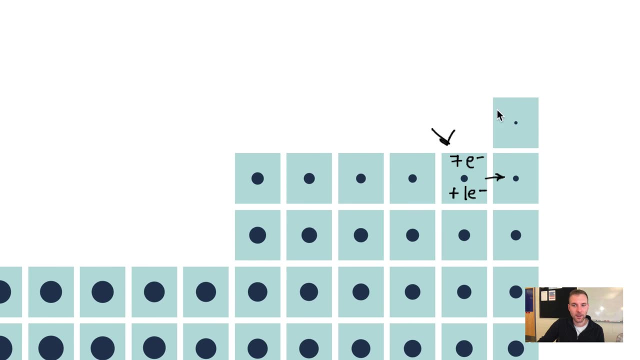 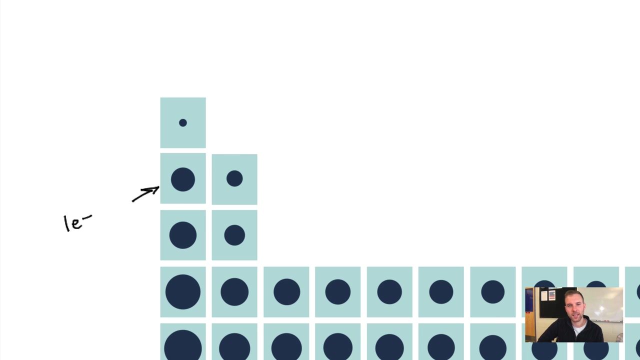 Lithium has one valence electron and does not want to gain any more valence electrons. In fact, lithium would actually prefer to lose that one valence electron to become a lot like helium, And so the electronegativity for lithium, for all the elements on sort of the left side of the periodic table, is going to be far lower. 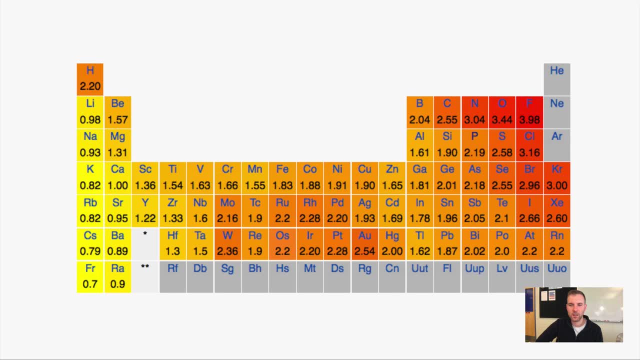 So let's take a look at just a special periodic table that only shows the electronegativity values. If I'm yellow, I really don't want electrons in this periodic table, And if I'm red that means I really do. Again, let's look at fluorine: 3.98 compared to lithium's 0.98.. 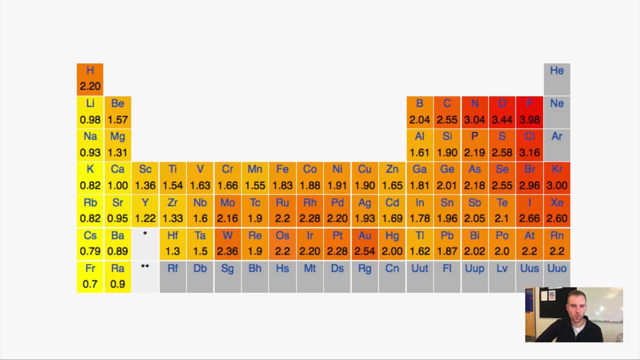 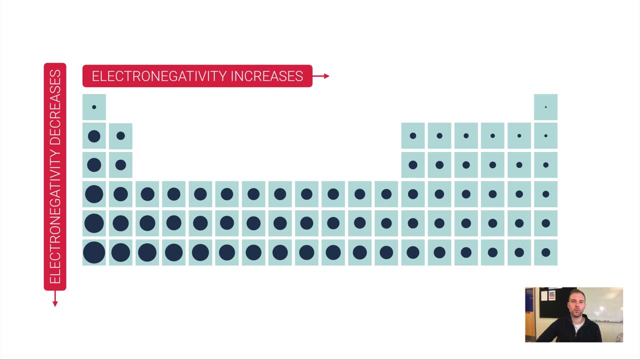 There it is, And so if I just kind of look from left to right within a period, I'm going to see that the electronegativity increases. If I go top to bottom in a group, the electronegativity actually decreases. 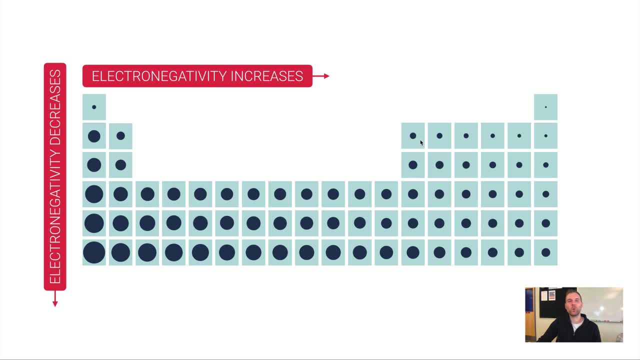 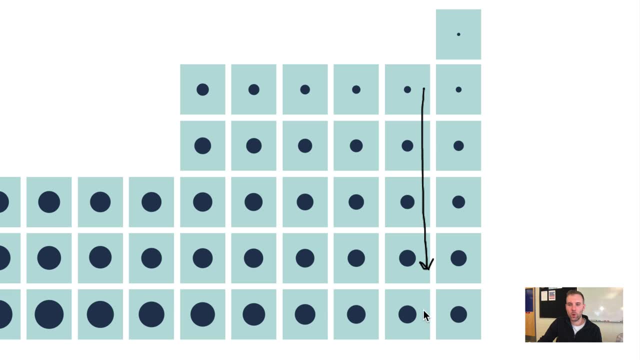 And this again, unsurprisingly, has a lot to do with the radius of the atom. If I just kind of look kind of down this way here, all of these halogens would like to gain one electron, to be like their noble gas neighbors. 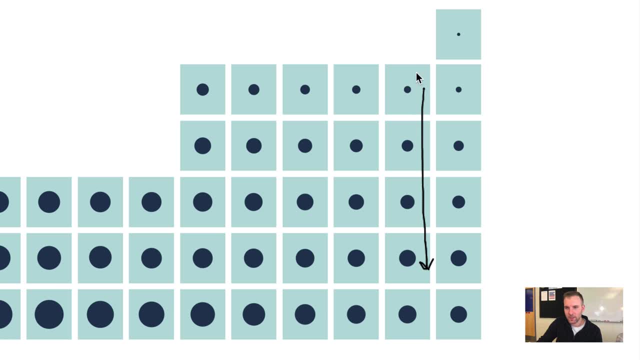 It is much easier for fluorine to attract an electron that isn't originally its own. because fluorine is so small, Its nucleus is located very close to the atom. It's very close to its valence shell. As you go from top to bottom, the nucleus gets further and further tucked in the center. 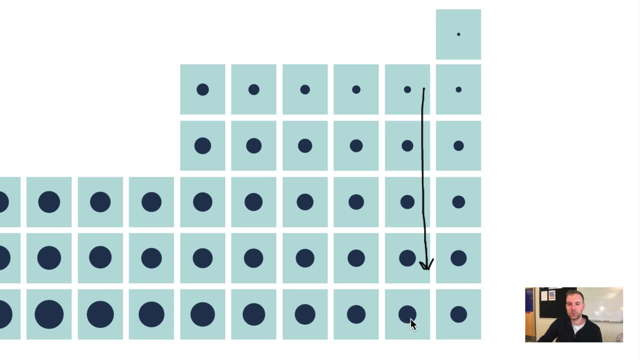 The valence electrons get kind of further and further out. So the electronegativity actually is a little bit lower as we go top to bottom, not because they don't want that one electron, but because their pull on neighboring electrons is a little lower because they're just bigger atoms. 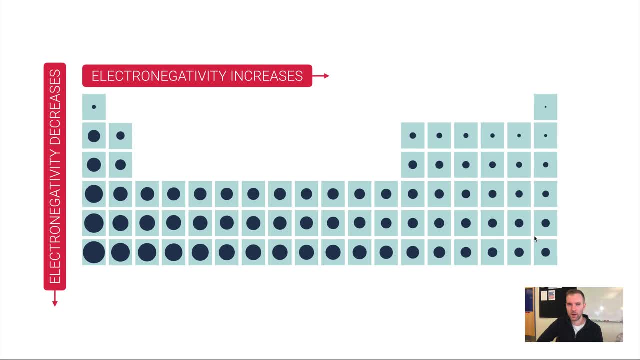 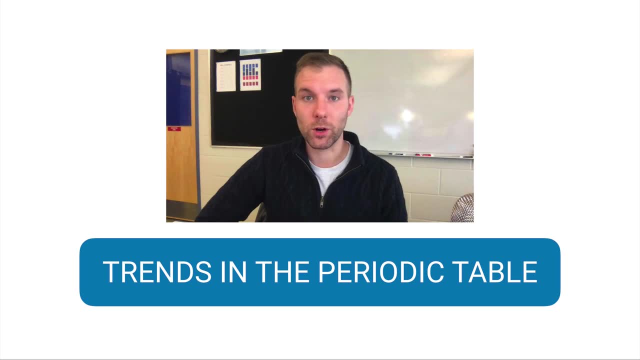 And so that's what's going on top to bottom in a group on the periodic table for electronegativity. So that's it. Those are the three trends in the periodic table. It's important that you know what the trends are for sure. 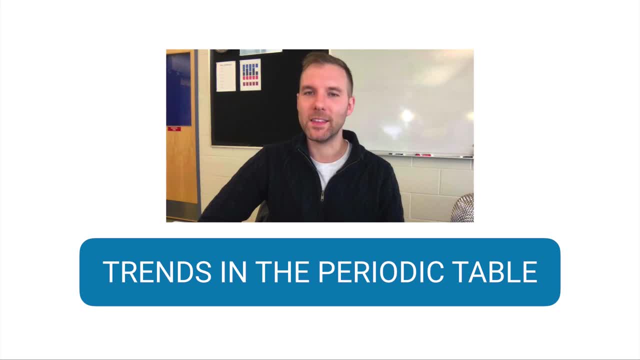 but I believe it is way more important that you know why these trends exist, And if you think about it long enough, it really all boils down to the size of the atoms. In many cases it's about the distance between the nucleus and the valence electrons. Thank you.